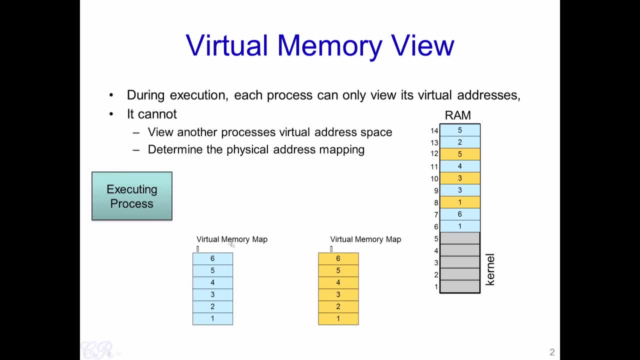 it sends out virtual addresses, which get sent out, It gets mapped into this virtual memory map and we had seen that there is an MMU which uses page tables stored in the memory and converts these virtual addresses into physical addresses. Now we have also seen that each process that executes in the CPU will have 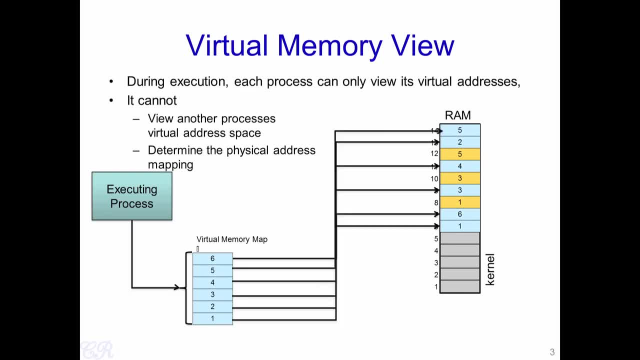 its own virtual memory map. The use of virtual memory map provides some level of abstraction. The executing process would only know its virtual addresses and with that virtual addresses it can only access the user space of the virtual memory map. So we had seen that the MMU then. 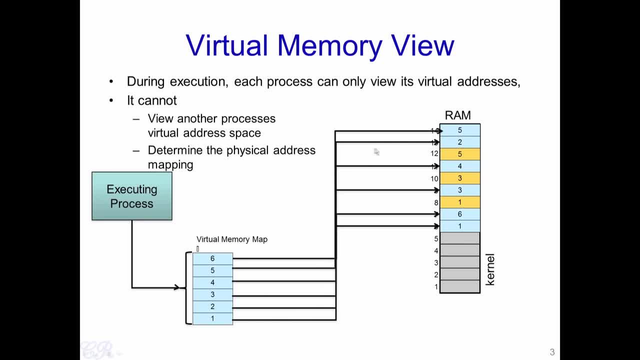 transfers this mapping into corresponding physical addresses. So the executing process will have no way to determine what the corresponding physical address for its memory accesses are. So, for instance, if you declare an integer i in your program, you can print out the virtual address corresponding. 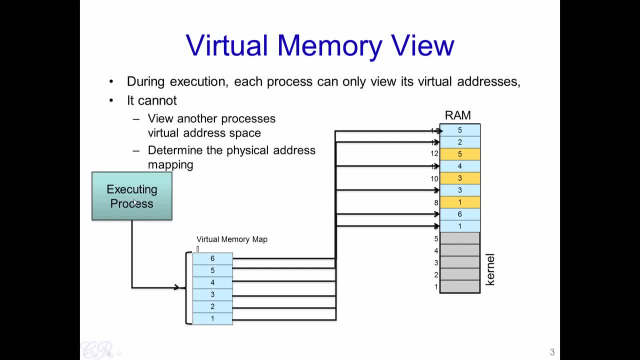 to i, for example with printf ampersand i. However, it is not possible for you in the user space to determine what the corresponding physical address is for that particular variable, i. The second thing: what the virtual memory map provides is that the executing process can. 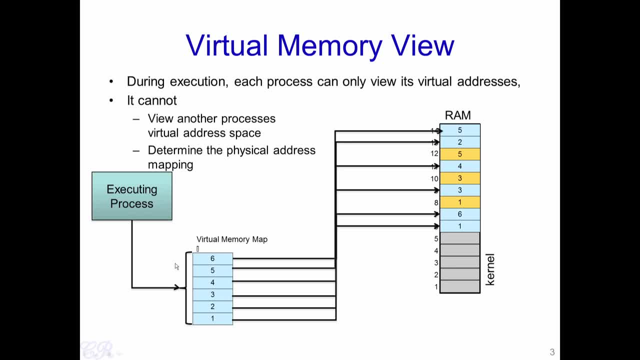 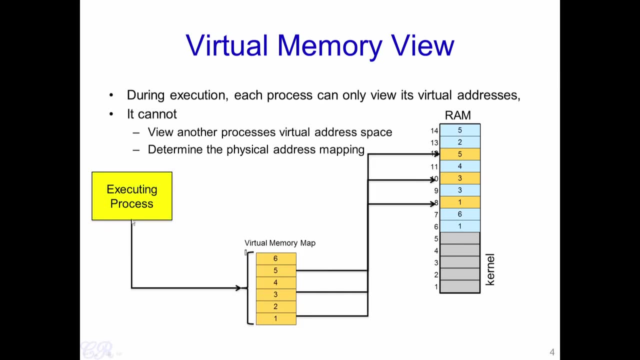 only have access to its own virtual memory map. So if there is another process it has with its own table now in user space there is no way for the executing process to determine anything of the other process. So when there is a context switch and a new process executes, it is the second process's virtual address. 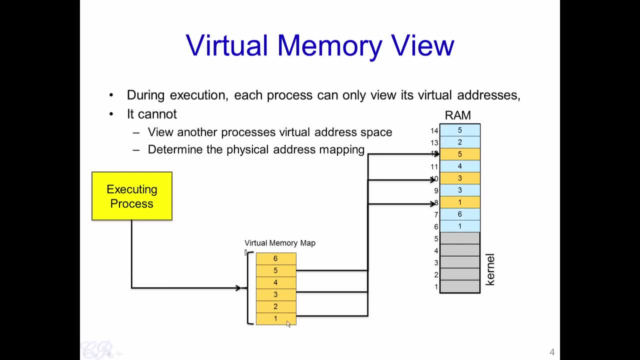 map or virtual memory map which is then used. So this process has no way to determine any other process's virtual address map. from these two slides is that a process has no way to determine any information or any data about an other process. 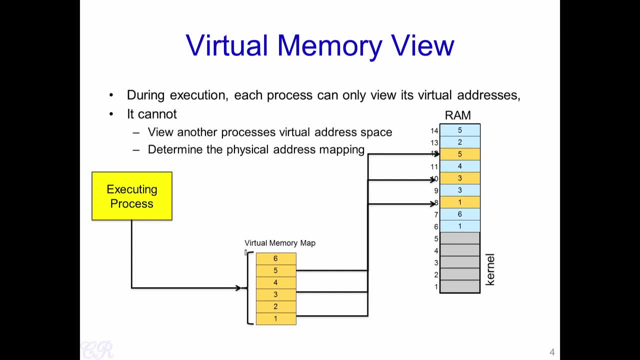 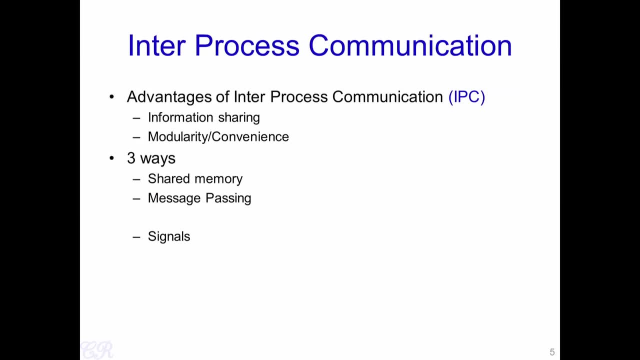 So, given this, how does one process communicate with an other process? So, in order to do this, there is a mechanism known as inter-process communication. Essentially, with IPCs or inter-process communication, two processes will be able to send and receive data between themselves. 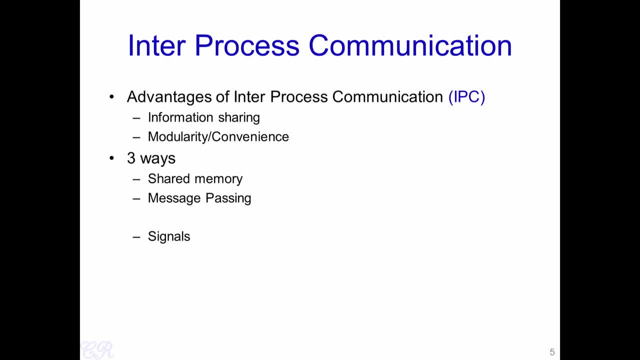 The advantage of IPC is that the processes could be written to be modular, So essentially, each process is meant to do a single job, and a processes could then communicate with each other through IPCs. For an example, let us say we have a data acquisition system and a control system. 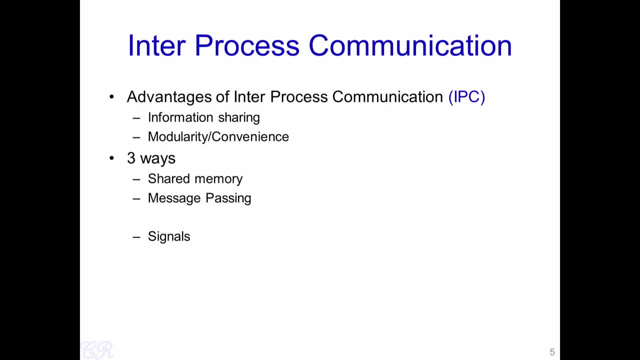 So, essentially, we could write one process which acquires data from the IPC, The external world, such as the temperature, pressure or the speed, and then it could then send this information or the data collected to a second process which then analyzes the data and determines some particular parameters. 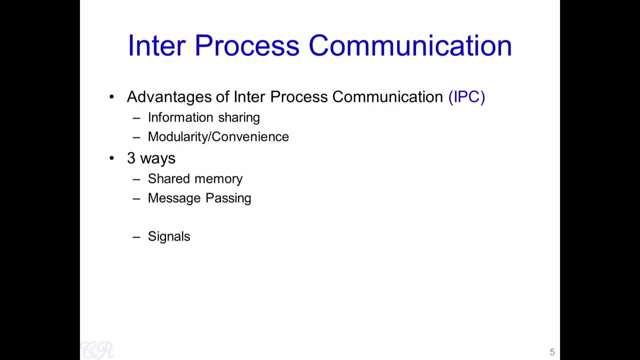 So these parameters could be sent to a third process which then actuates some external data. For instance, it could open a valve or close a valve, It could adjust the temperature of the room, and so on. Thus we see, we are able to achieve a modular structure in our application. 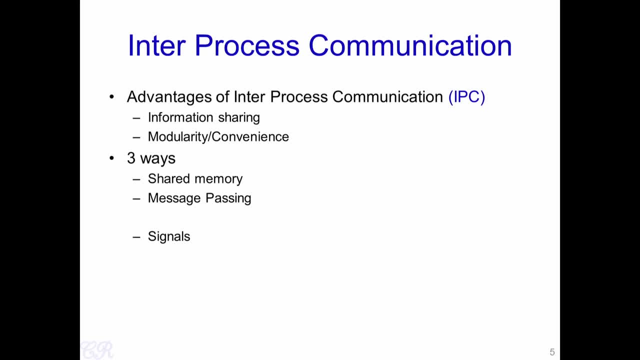 Each processes job is to only focus on a single aspect. The communication between the processes is achieved by inter-process communication. In typical operating systems, there are three common ways in which IPCs are implemented. These are through shared memory, message passing and signals. 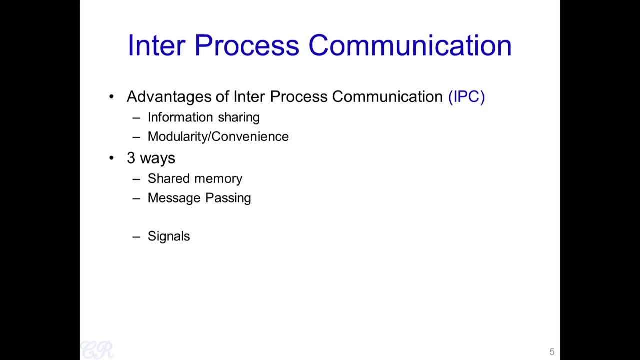 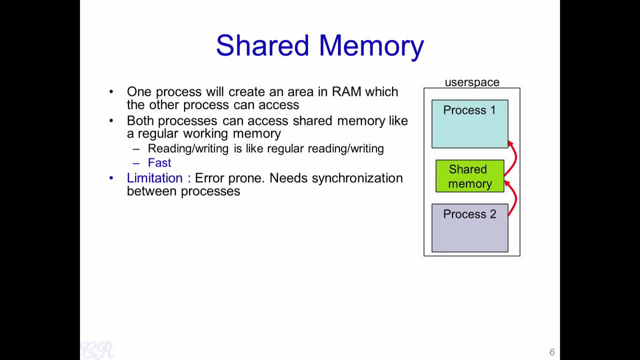 So this is the process. So let us look at each of these things. So, with the shared memory, we have one process which creates an area in RAM which is then used by another process. So essentially, the communication between process 1 and process 2 is happening through. 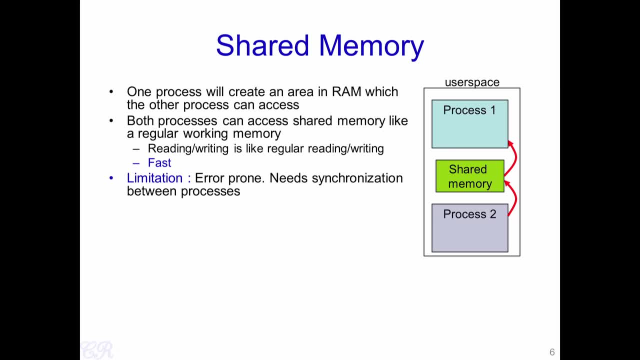 this particular shared memory. Both processes can access the shared memory like a regular working memory, So they could either read or write. So they are all connected to this particular shared memory independent of each other. The advantage with this is that the communication is extremely fast. 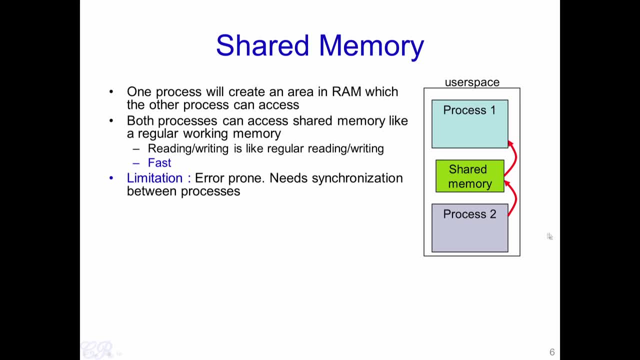 There are no system calls which are involved, and the only requirement is that you could define an array over here and then fill the array in the shared memory, which can then be read by the other process. The limitation of the shared memory approach is that it is highly prone to error. 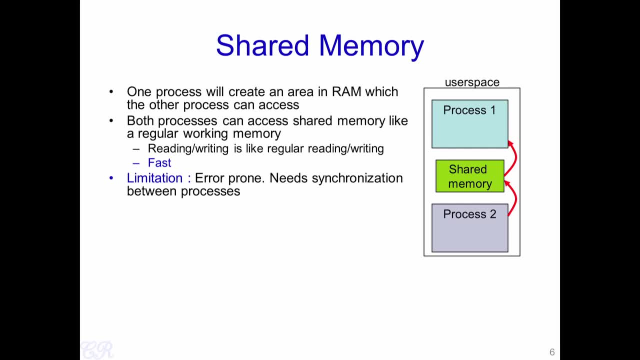 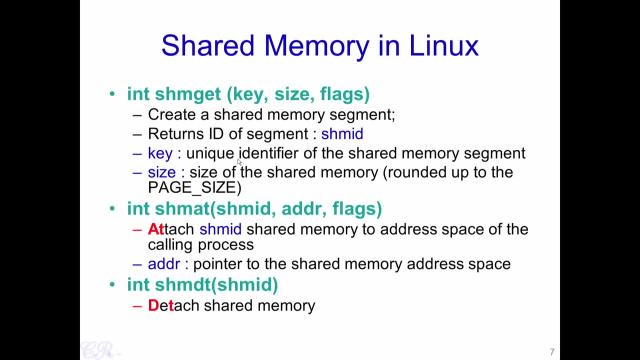 prone to error. it requires the two processes to be synchronized. So we will take a small example of how shared memory is implemented in Linux. So essentially in shared memory in the Linux operating system we have three system calls which are used. 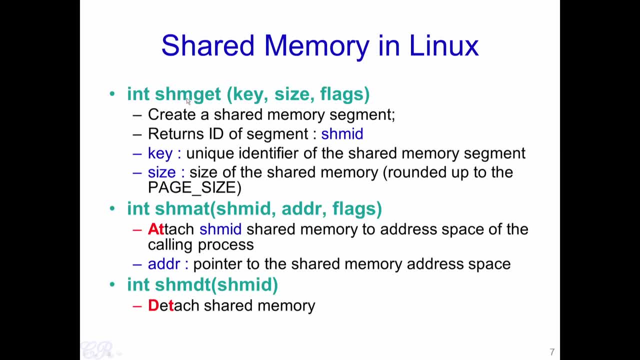 First is the SHM GET or the shared memory GET, which takes three parameters: a key size and flags. So this system call creates a shared memory segment. It returns an ID of the segment, that is, SHM ID, the shared memory ID of the segment. 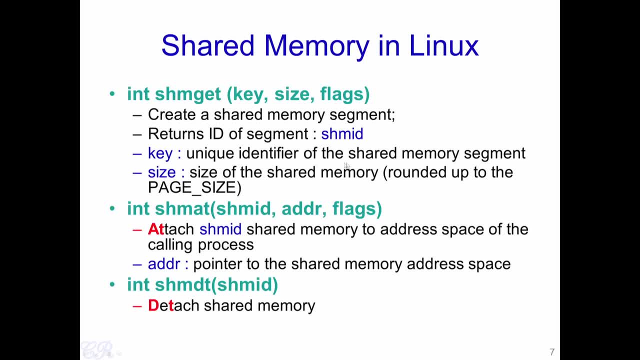 So the parameters key is a unique identifier for that shared memory segment, while size is the size of the shared memory. So this is typically rounded up to the page size. that is 4 kilobytes. So this is how a shared memory gets created in a particular process. 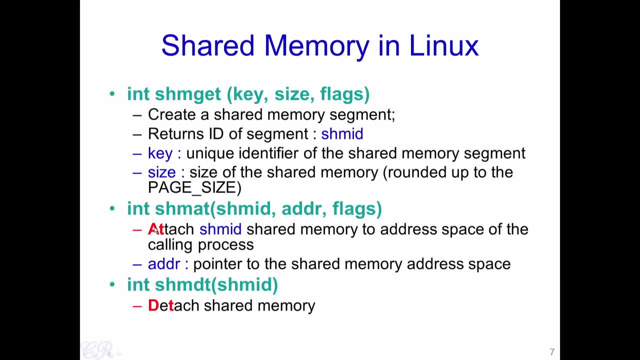 Now an other process could attach to this shared memory by this particular system call, that is, shared memory, attach SHM AT. So this particular call requires the shared memory ID and address and flags. So essentially, system call would attach a shared memory to the address space of the. 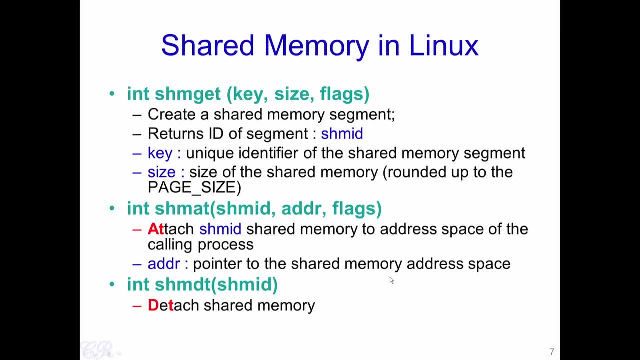 calling process. The address is a pointer to the shared memory, So the shared memory is the shared memory address space. So we will understand more of this through an example. The opposite of the shared memory attach is the shared memory detach where a process could. 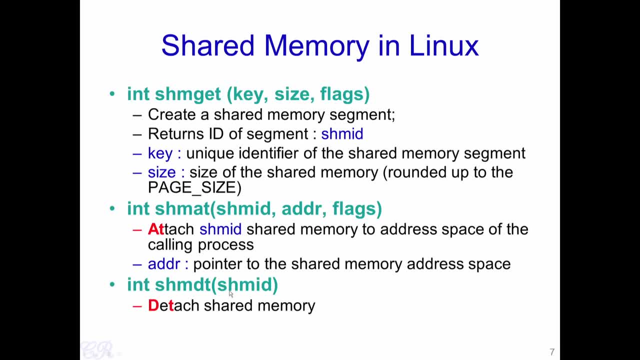 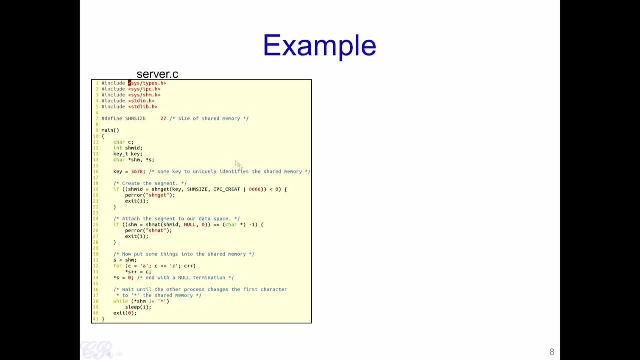 detach the shared memory from its user space. So the detach system call takes the shared memory ID. Let us see the an example of shared memory with this example. So let us say we have written this particular program called server dot c. So let us say we have written this particular program called server dot c and we create a. 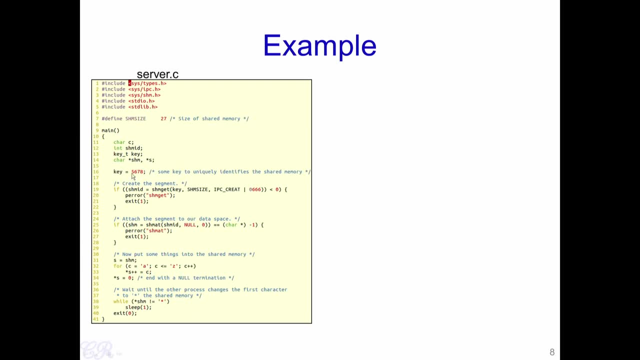 shared memory in this, So we define a key called 5678.. This is some arbitrary value for key, but the requirement is that this key should uniquely identify the shared memory, So we could use this key to invoke this function: SHM GET. 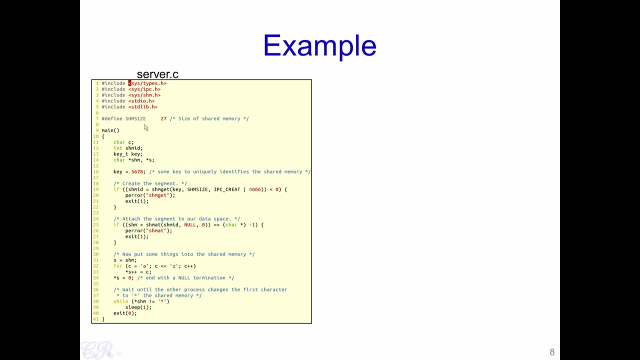 We pass it the key. we pass it SHM size. that is, SHM size is defined here as the size of the shared memory. This is the size which we want to create. Note that this size, although we specified as only 27 bytes, will get extended to a page. 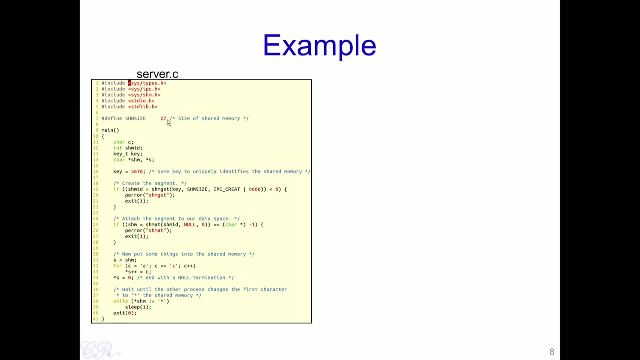 that is, we will create a page of 4 kilobytes corresponding to this. The third parameter is the permissions, that is, we are given it as IPC create, that is, we are creating this particular shared memory and these are the permissions: read, write, execute permissions. 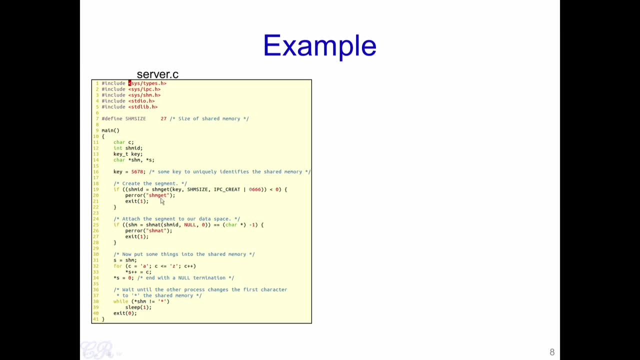 And, of course, if this, If this function fails, then it enters over here and exits. otherwise, if it executes successfully, we get a valid shared memory ID. The next part is to invoke the shared memory, attach SHM AT providing this particular ID and we will get a pointer to this particular shared memory. 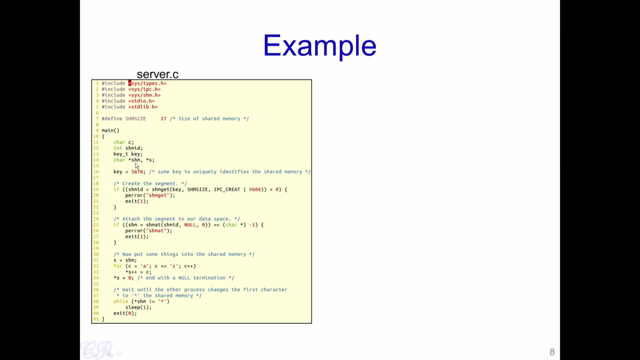 So SHM. so we have, like char star, SHM. this is a pointer to the shared memory. Now the shared memory attach would return a pointer to this particular shared memory. Now, in case it returns minus 1, then it is due to an error and we are exiting. 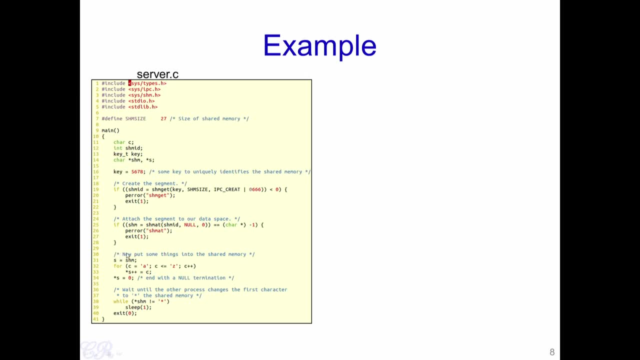 Now, at this particular point, we have obtained a pointer to the shared memory and we can use that particular pointer just as a standard pointer we as we use in a C program. So, for instance, over here we have moved the pointer to this variable s, which is defined. 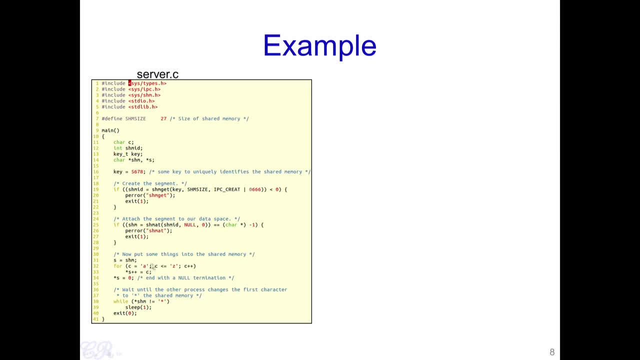 as char star s, and we have put alphabets from a to z in this thing And finally we have ended it with a null termination, and then we are going in a loop, continuously sleeping. So we will come back to these two statements later on. 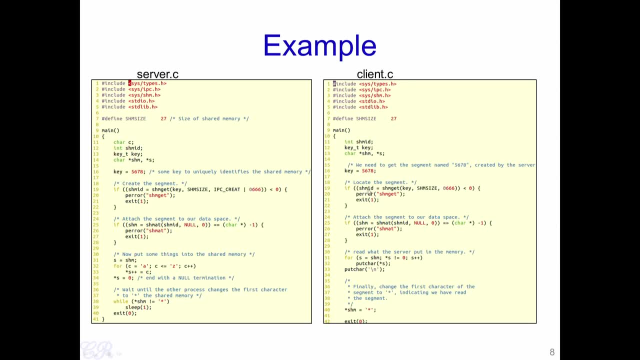 Now let us look at the client side of this code. So we invoke this SHM GET and give it the key. that is key is the same: 5678, the shared memory size It has before 27, and we are providing the permissions. 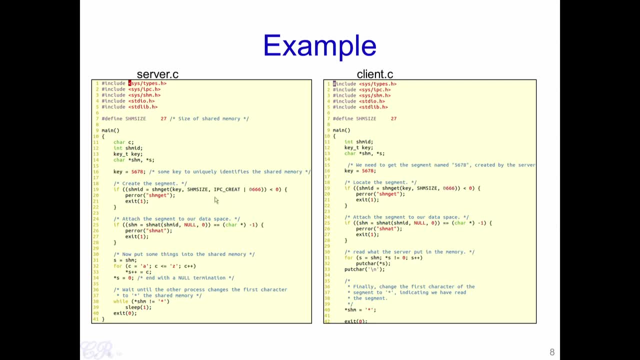 Note that we do not require to give create over here, because the shared memory region is already created. Then we attach to this particular shared memory segment as before we invoke the function shared memory. attach SHM AT and we pass it the shared memory ID. 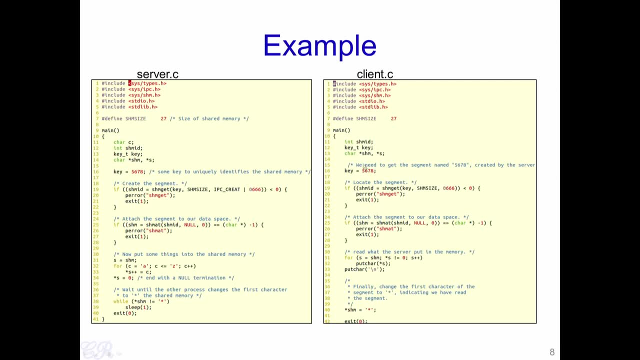 Then we get a pointer: SHM. So this is the SHM, which is a pointer to this shared memory location. So essentially, both the server as well as the client are pointing to the same physical memory page. Now we could actually read data from this particular shared memory region. 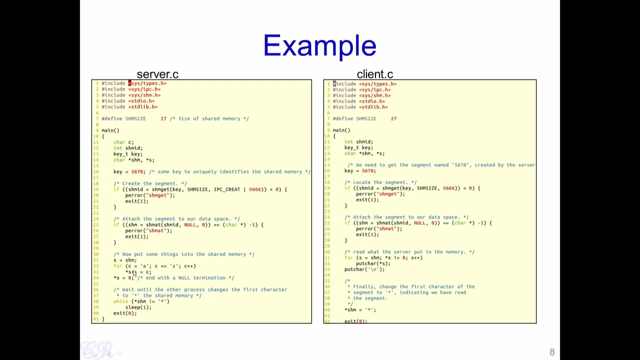 So remember that the server has put values from a to z, that is, a, b, c, d to z, while in this case we could read the values a to z into the shared memory region. So now we can see that the server has put values from a to z, that is, a, b, c, d to z, while 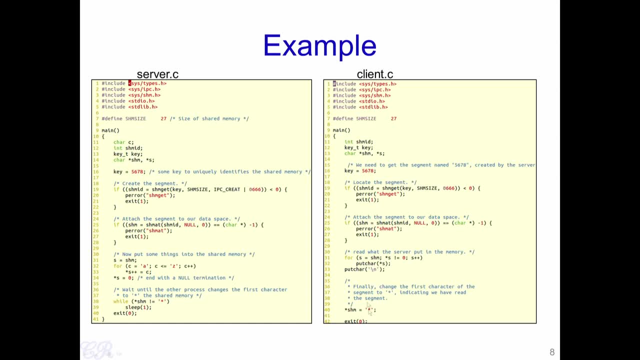 in this case, we could read the values a to z into this particular pointer s and print it out in the scheme. So once we have completed reading all data from the shared memory, we put this star into the shared memory location. This is the first location in the shared memory. 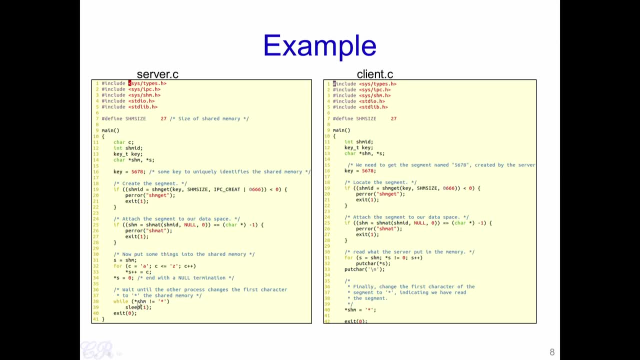 Now recall that over here in the server we have put a while loop which continuously loops until the first parameter pointed to in the shared memory is a star. So when we obtain a star, it means that the client has completed. 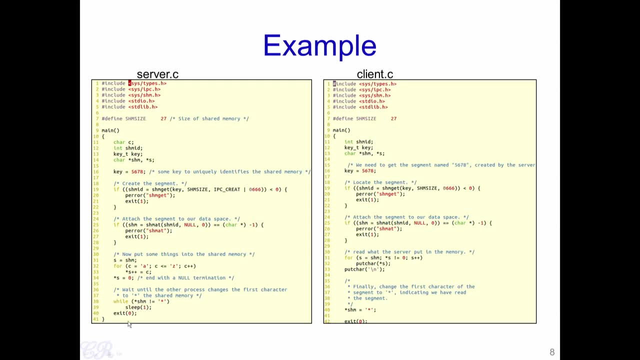 completed reading all data and therefore the server can exit. In a similar way, the client can exit as well. So you see that we have these two processes- one is server, one is client- and these two processes are having their own virtual address space, but by the use of the shared memory. 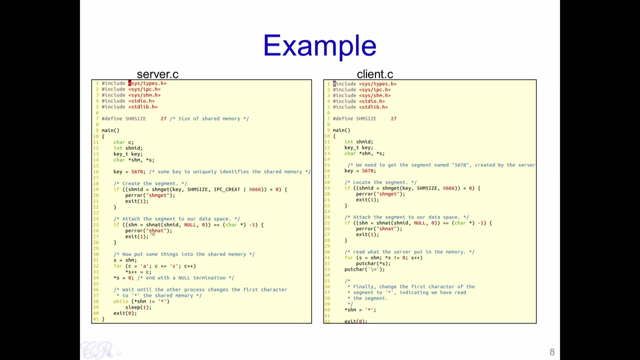 which is created by the shared memory gate and shared memory attach, we are able to create a shared memory region which is common between the server and the client. Then we have obtained a pointer to that particular shared memory region. that is S on SHM and. 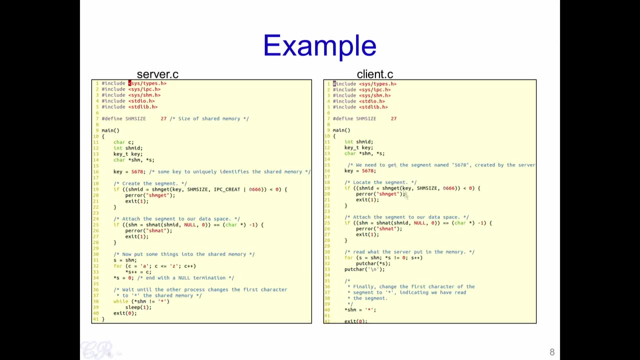 the server could put data into that shared memory region, while the client could read data. the vice versa is also possible, And at the end of it we require to note that there is a synchronization required between the server and client, So this synchronization requirement should be explicitly programmed into this particular. 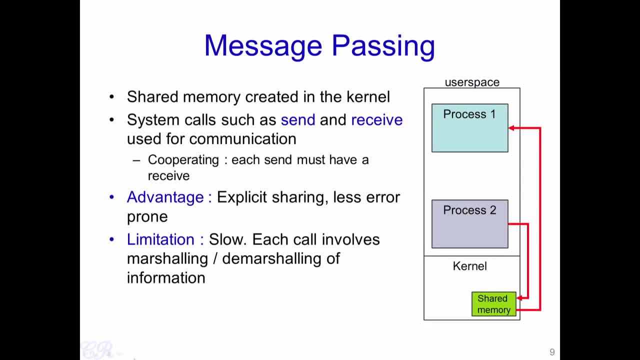 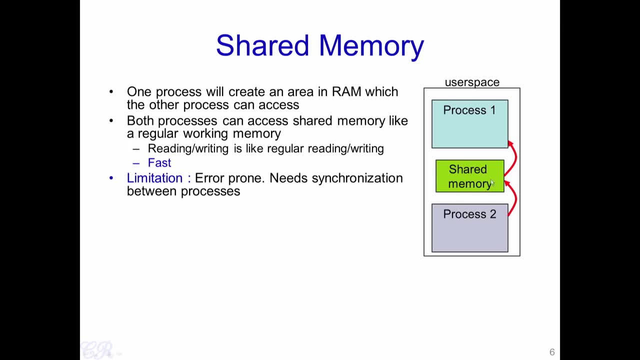 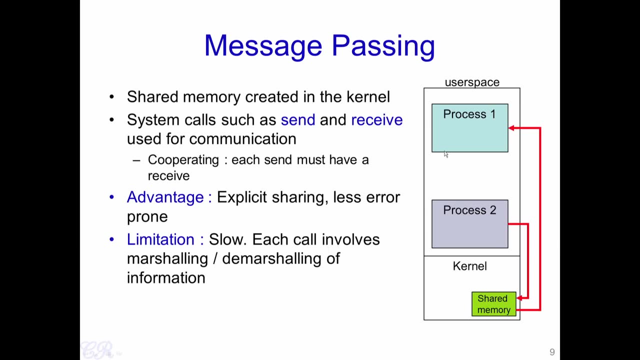 server client modules. Next, we will look at the message passing. Unlike the shared memory that we just seen, where the shared memory is created as part of the user space in message passing, the shared memory is created in the kernel. Essentially, we would then require system calls, such as send and receive, in order to communicate. 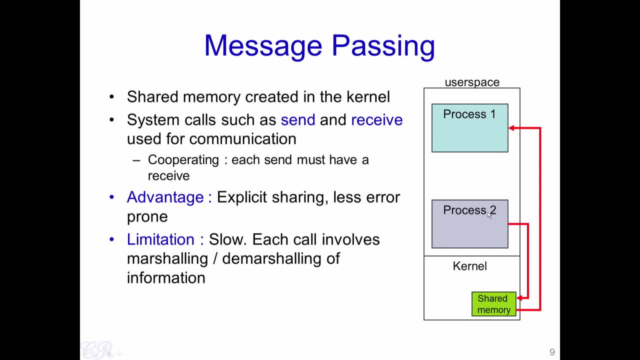 between the two processes. If a process 2 wants to send data to process 1, it will invoke the send system call. So this would then cause the kernel to execute and it would result in the data written into the shared memory, while, when process 1 invokes, receive data from the shared memory would. 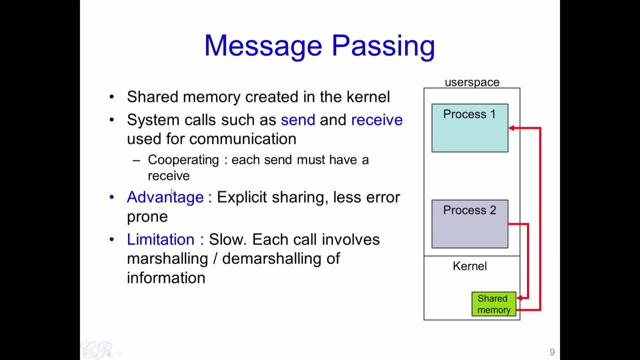 be read by process 1.. The advantage of this particular message passing is that the sharing is explicit. essentially both process 1. And process 2 would require support for the kernel to transfer data between each other. The limitation is that it is slow. 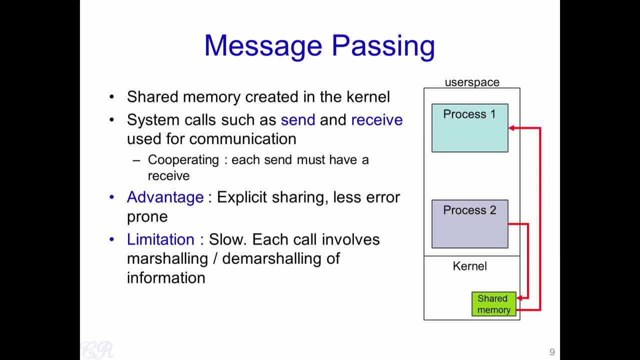 Each call for the send or receive involves the marshalling or and demarshalling of information And, as we know, in general a system call has significant overheads. therefore, message passing is quite slow. compared to shared memory, However, it is less error prone. 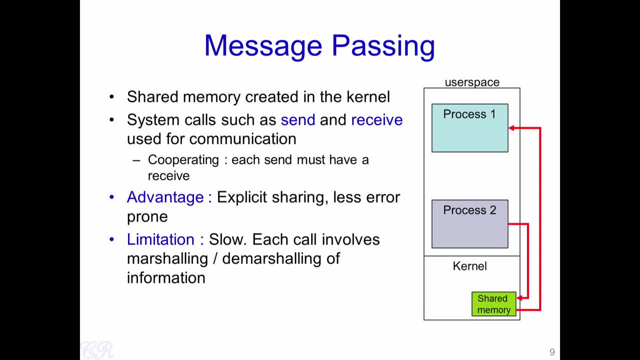 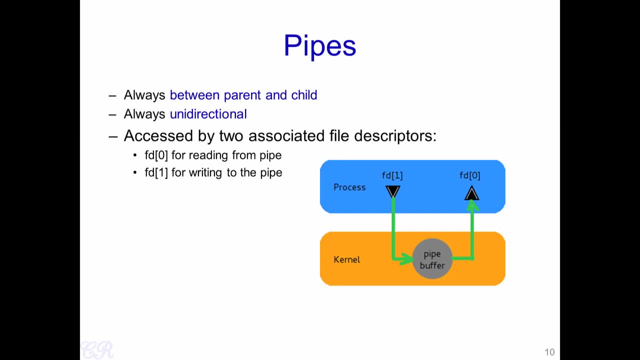 Then shared memory, because the kernel manages the sharing and therefore would be able to do the synchronization between the process 1 and process 2.. Another very common application of message passing is the use of pipes. Now pipes are used between parent and child processes only. 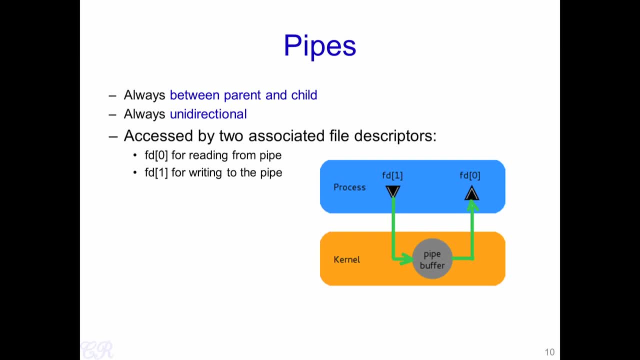 Essentially, you can only communicate data from a parent process to a child process and vice versa. Another aspect of pipes is that it is unidirectional. Now, when a pipe is created, generally there are two file descriptors which are associated with it. that is, FT0, which is used to read from the pipe, while FT1 is used to write to. 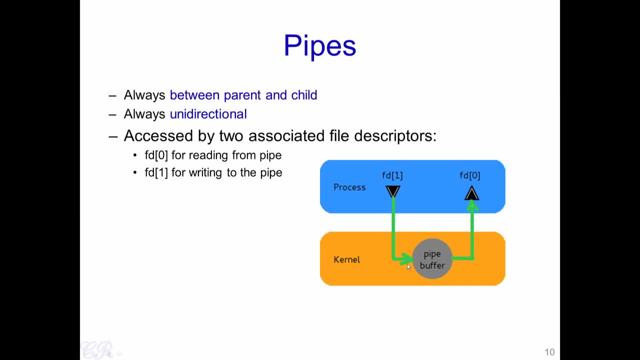 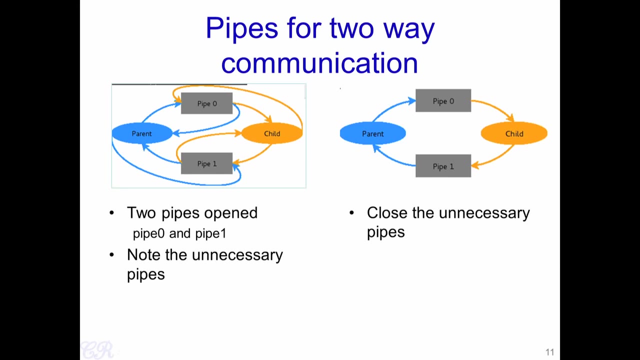 the pipe. So we know the unidirectional nature of this particular IPC. So FT1 is exclusively used to write to the pipe buffer, while FT0 is used to read from the pipe buffer. So in order to obtain two way communication between the parent and the child, we would 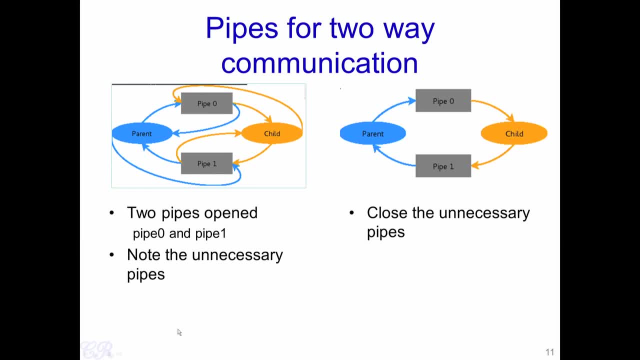 require two pipes to be obtained: pipe 0 and pipe 1.. So when pipe 0 is opened, it would create two file descriptors, one to write into pipe 0 and the other one to read to from pipe 0. Similarly, there are two file descriptors to write to pipe 1 and read from pipe 1.. 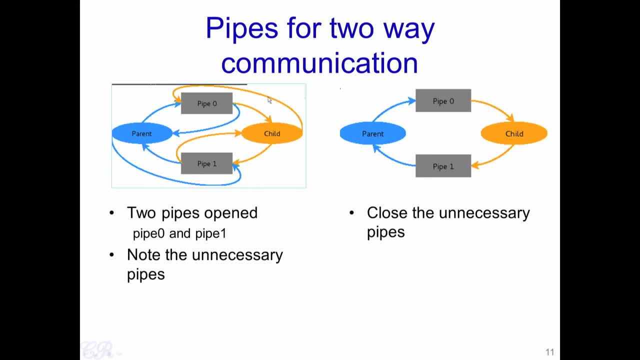 Basically, there are two pairs of file descriptors for pipes in the child process. Now you note that these additional descriptors are not required. Therefore, it we could actually close the extra file descriptors to obtain something like this Now, in order that the parent sends some information to the child. 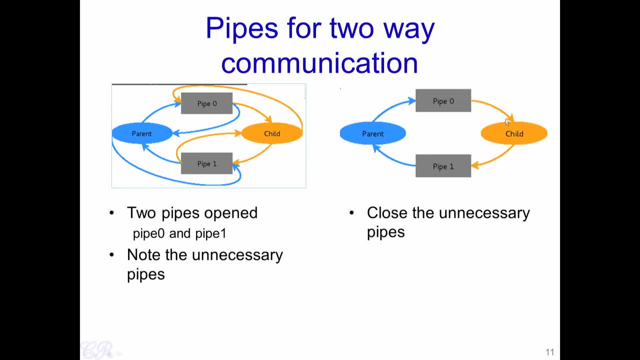 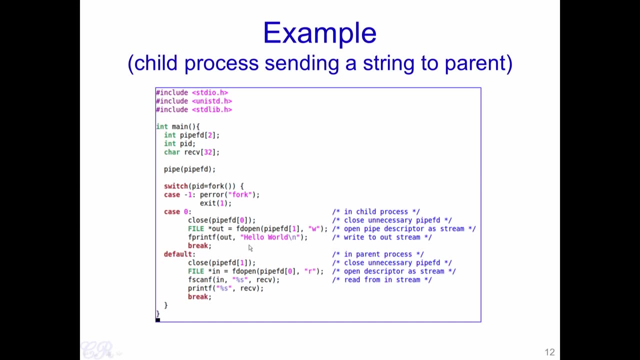 The parent will write to pipe 0, while the child will read from pipe 0.. In order to that, the child sends some information to the parent. the child will write to pipe 1, while the parent will read from the pipe 1.. So let us see an example of the use of pipes. 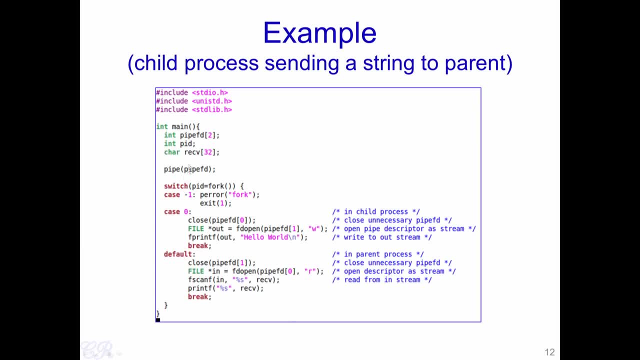 So this again is a standard Linux example and, as we have said so, we create a parent and child process so that there is a unidirectional communication from the parent to the child. So let us look at this particular thing. First, we invoke this particular system call called pipe and give it this pipe fd. 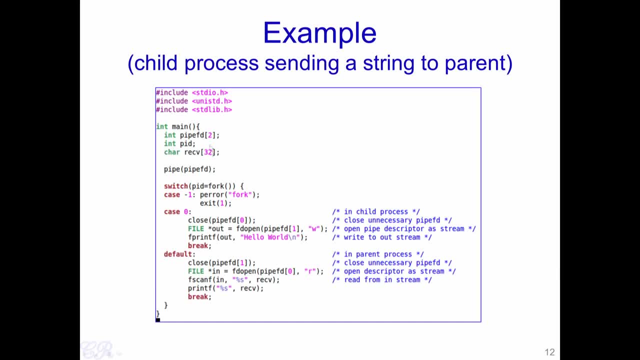 So pipe fd is defined over here and taking two elements. and then we invoke the system call, fork. So as we have studied the fork system, call would create a child process which is the exact duplicate of the parent process. So in the parent process the value of a pid, that is the value what fork returns, is the. 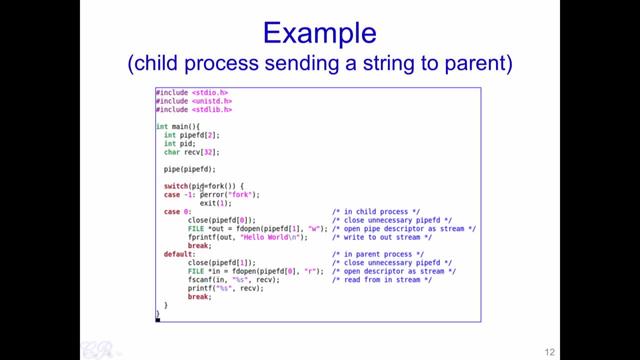 child's pid value, and it is a value which is greater than 0.. On the other hand, in the child process, the value returned by fork is 0.. So let us see what happens in the child process first. So, in the child process, because the pid value 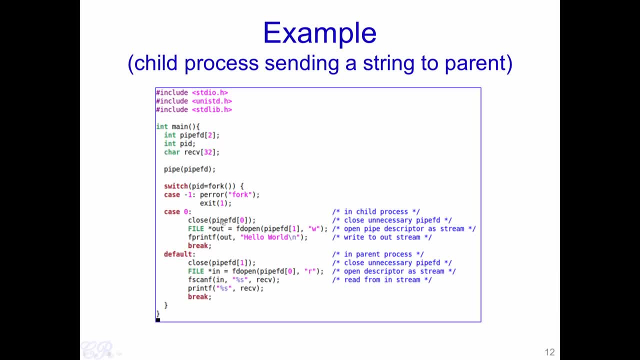 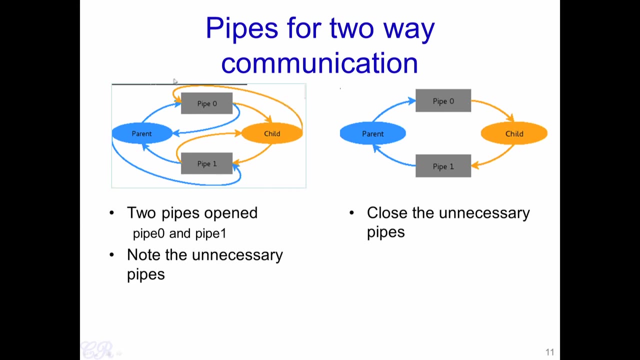 is 0. So it would come over here and the first thing what we do is we close pipe fd 0. So closing pipe fd 0 would mean that we are closing the read pipe to the child, that is. so we are having like two pipes over here corresponding to pipe 0 and we are just closing. 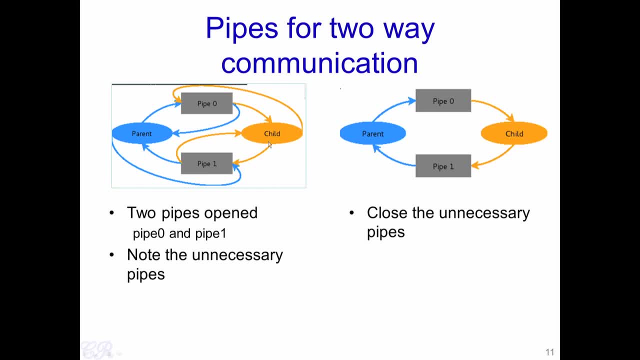 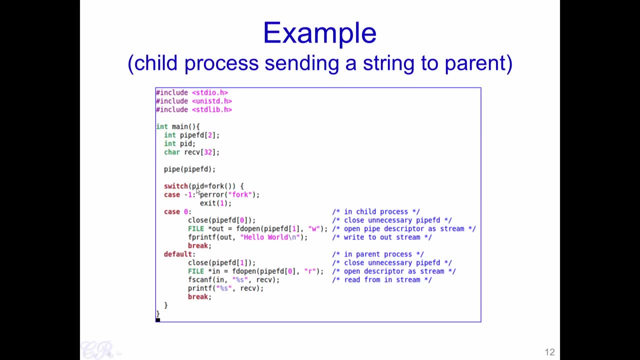 the read pipe, while the pipe 1, that is, the write file descriptor, is still open. Now let us see what happens In the child process. the value of pid returned by fork is 0. therefore, it will result in this particular code being executed. 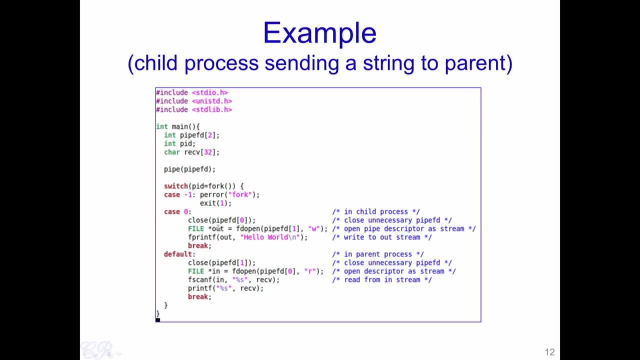 So in this code, first there is we are closing the pipe fd 0. So this means that the file descriptor corresponding to the read pipe is closed. Second, we are then opening a second file called fd open, corresponding to file descriptor 1, and it is open. 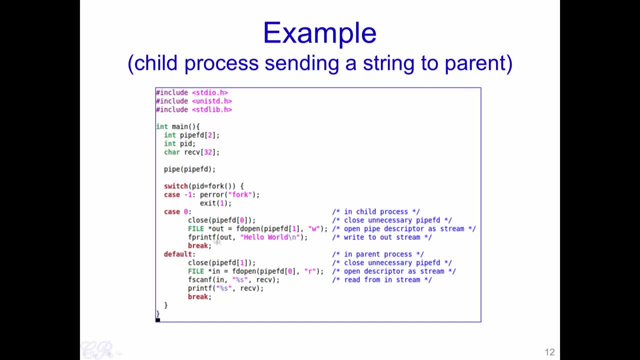 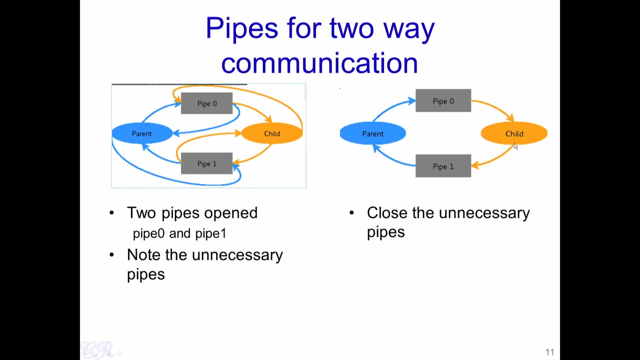 It is open in the write mode and we could then use fprintf out hello world. So essentially, what we are doing is to this pipe with descriptor 1, we are writing hello world. So if you go back to this particular thing, so what we are seeing is that we are writing. 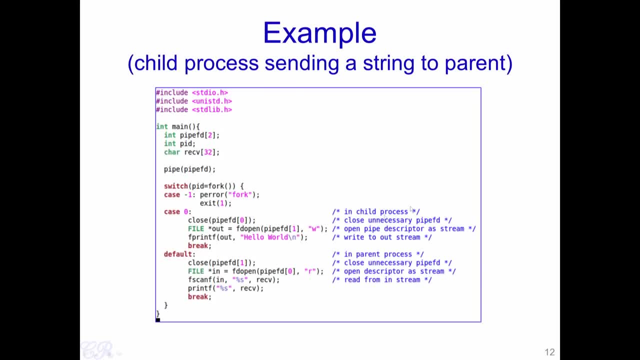 hello world, into this pipe. 1. Now in the parent process, which would execute over here because fork would return with a value. So we are closing the write pipe and opening, using fd open the read pipe. So we are then using fscanf to read whatever has been pushed into the pipe. in this case, 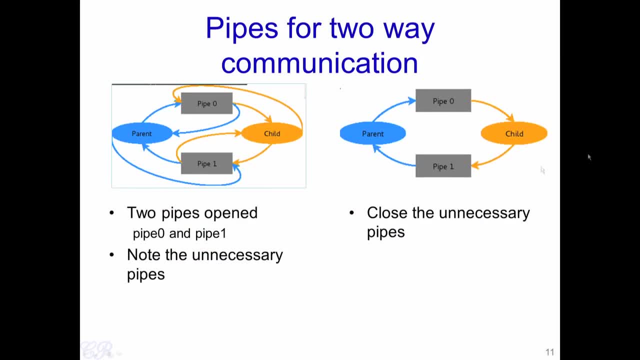 it is hello world and printing it to the screen. So essentially what we have implemented in this in the program is this lower part. So the child opens this pipe in the write mode and puts hello world into this pipe, While the parent then opens the pipe 1 in the read mode and reads the string hello world. 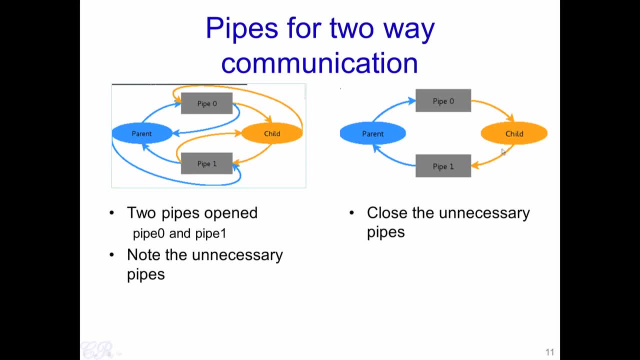 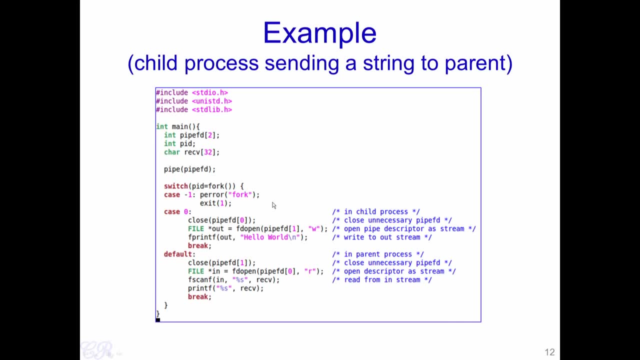 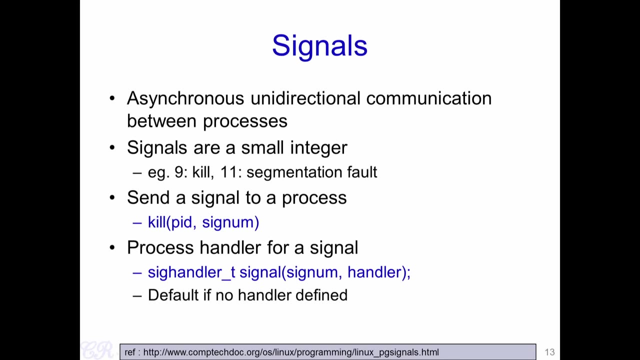 from the pipe. Thus the string hello world has been transferred from the child to the parent, So you can actually try to implement this particular program and execute in a Linux system, Besides the message passing shared memory and pipes that you have studied so far, a.